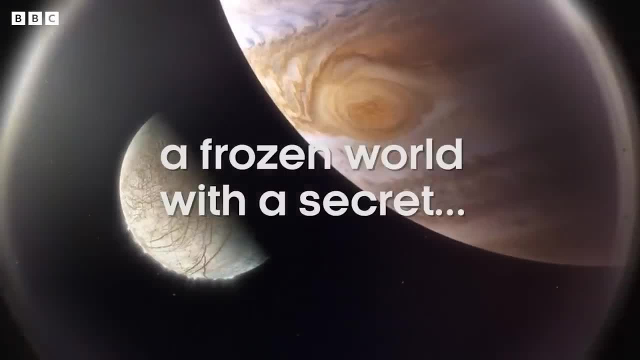 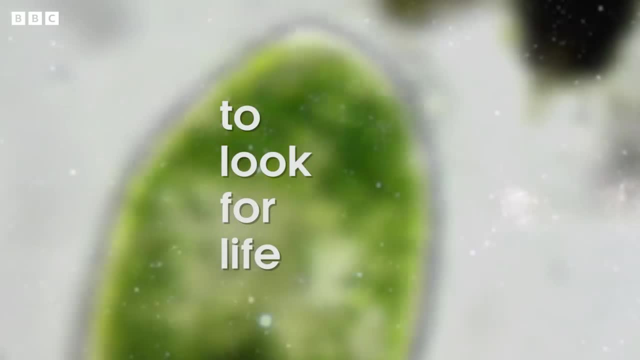 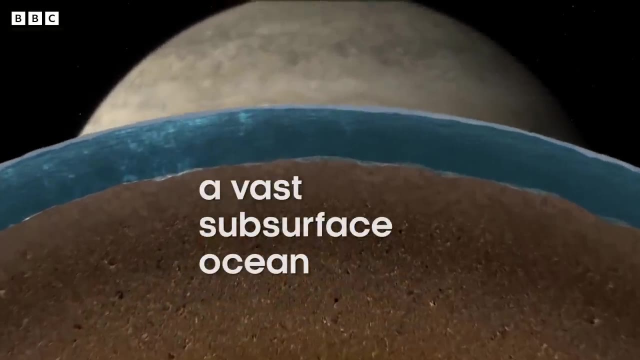 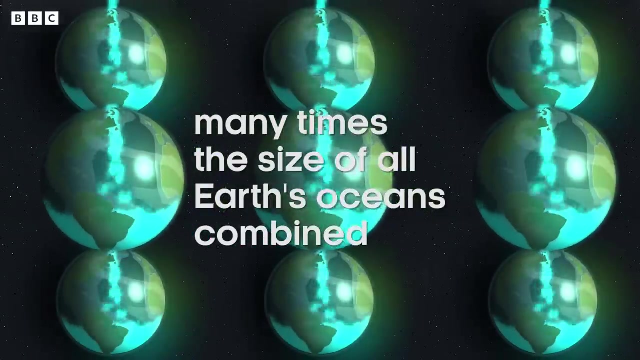 This is one of the few places in our solar system where we have a good chance to look for life. There's evidence for a vast subsurface ocean below the icy crust of the Moon. The amount of water that's suspected there is many times more than all oceans together we have on Earth. 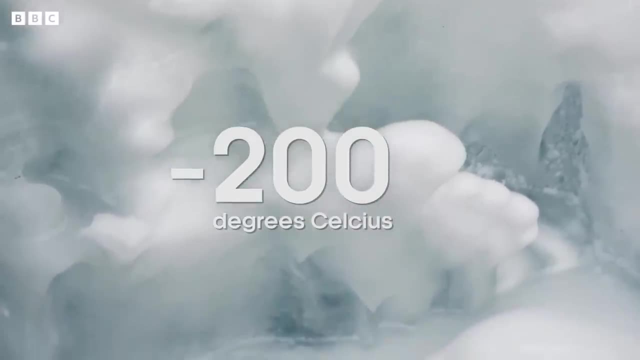 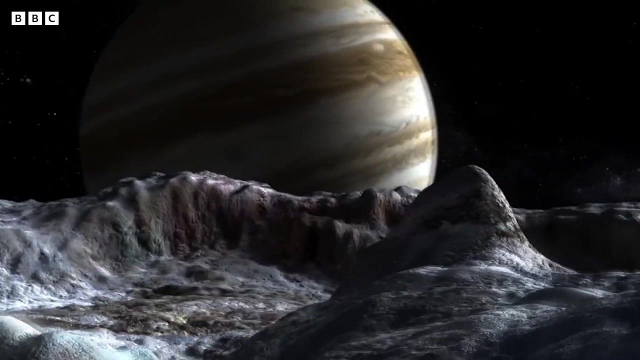 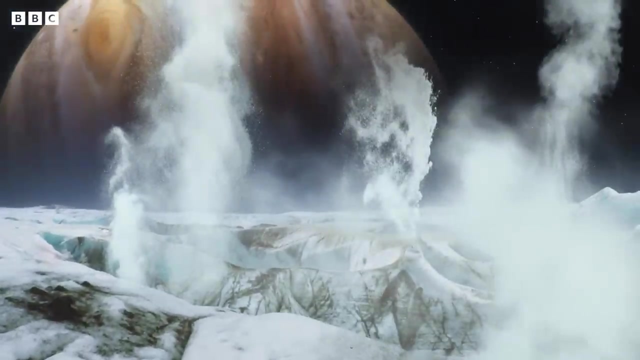 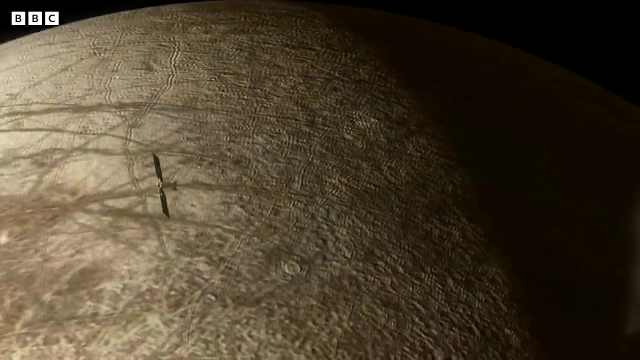 On the poles you're approaching minus 200 degrees Celsius. icicles that could be several meters high might be present, And if you're very lucky, then you might just spot a plume erupting nearby like an ice volcano that ejects material from the subsurface to enormous altitudes. 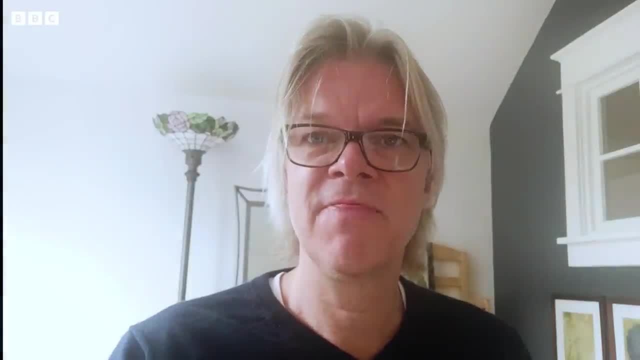 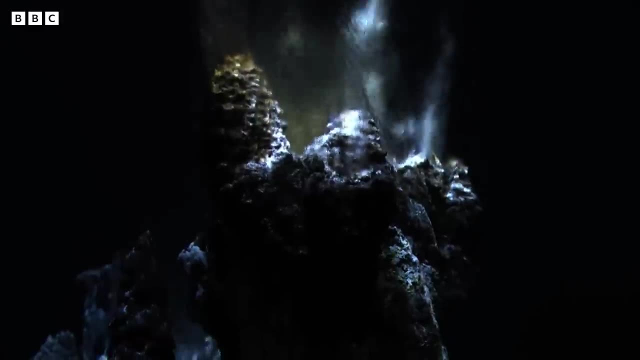 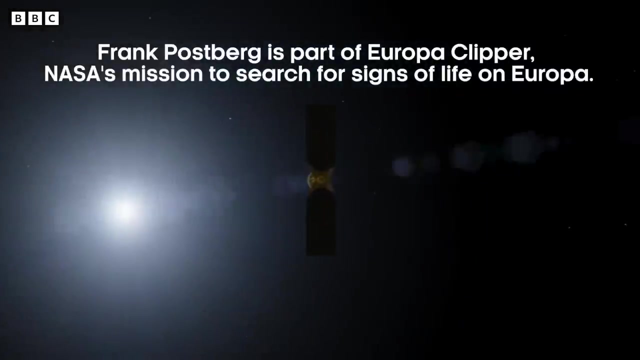 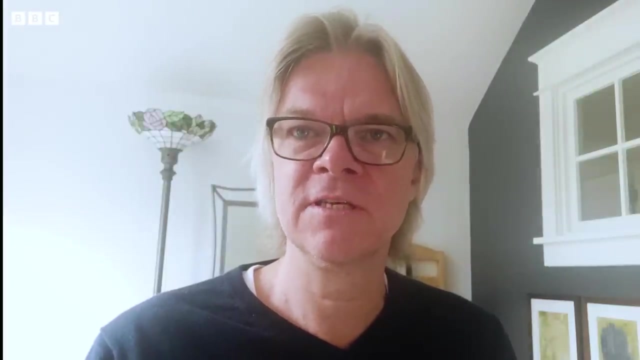 On top of that, there's a good chance that there's an energy source at the bottom of the ocean- hydrothermal activity- that can support the emergence of life. That makes Europa outstanding. Europa Clipper is the first mission that goes to the outer solar system. 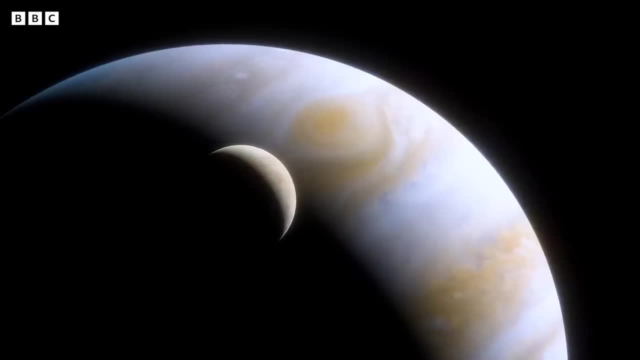 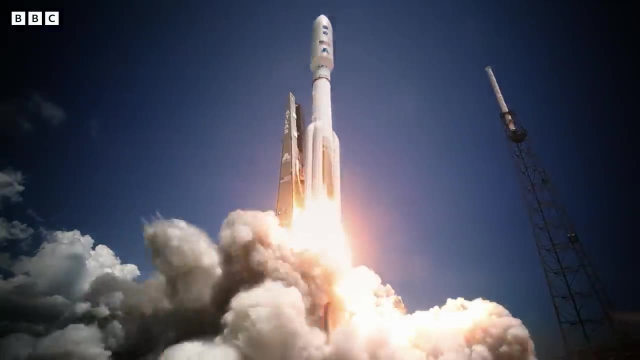 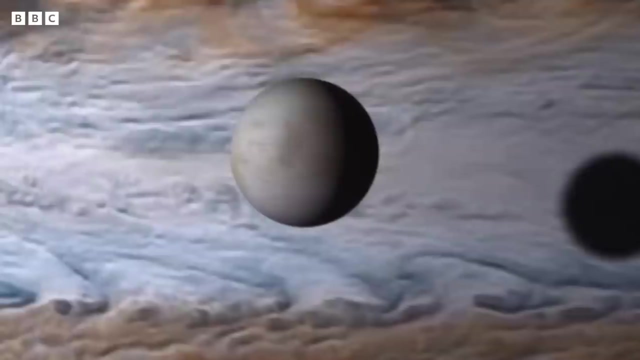 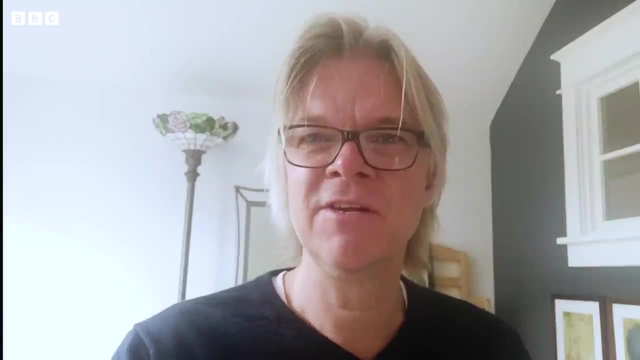 that has the exclusive goal to investigate the habitability of the body in the outer solar system. It will launch in October 24 and will arrive at Jupiter in April 2030. So it's five and a half years for Europa. Clipper Jupiter has about 70 moons, so the number increases every year by a bit. 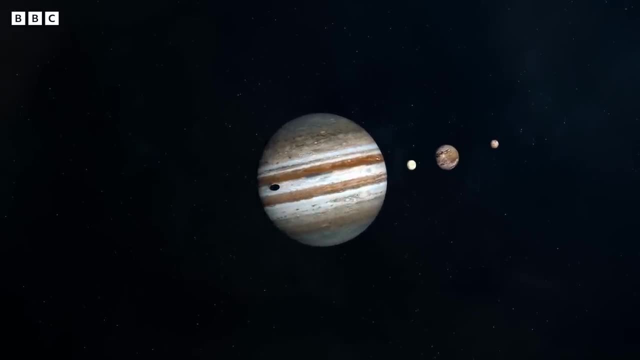 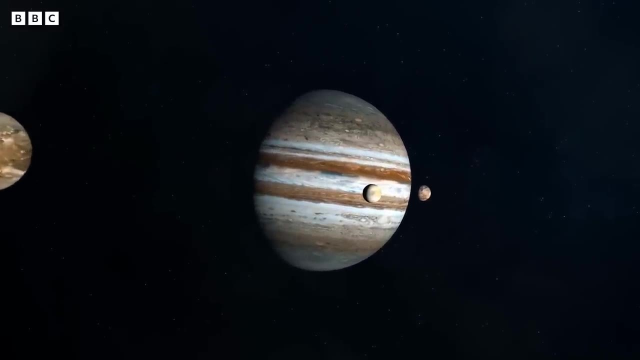 But there are four moons that stand out, That are the so-called Galilean moons. The innermost is Io, then Europa, then Ganymede and then Callisto, With the telescopic observations before the arrival of the first spacecraft. 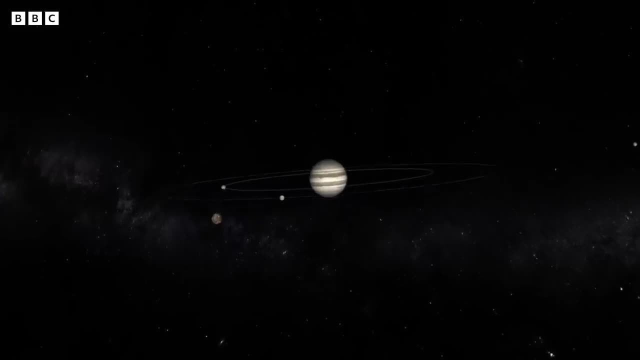 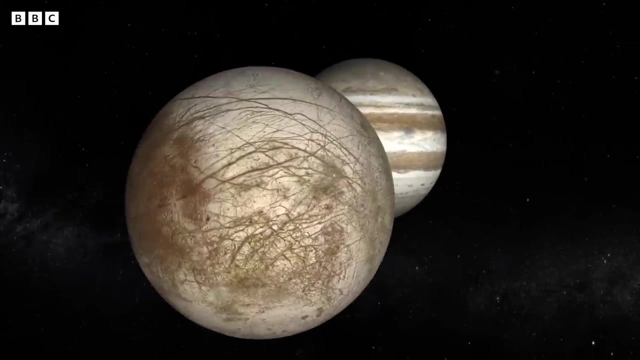 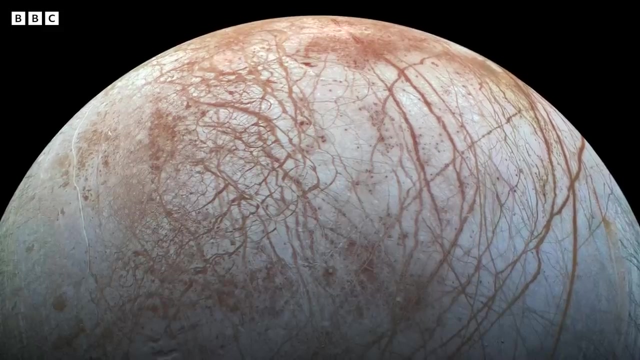 you could see that some of these moons are really really bright. They reflect way more light than a rocky surface would, And so, for example, Europa, and also Enceladus- they are one of the brightest objects, And so it was suspected already at that time that the surface might be composed of shiny, reflecting water ice. 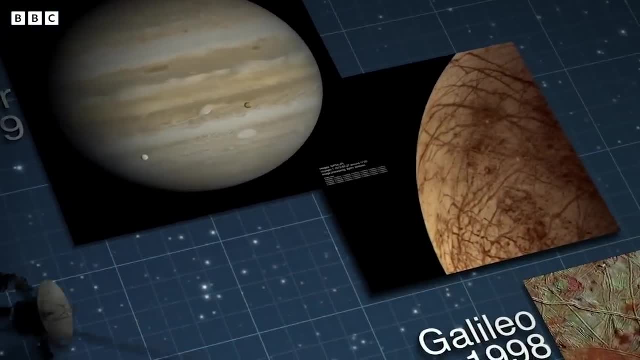 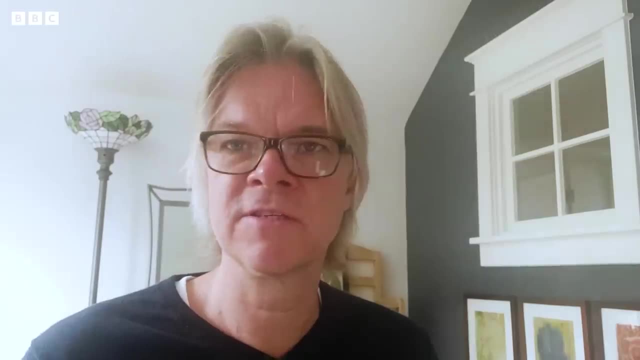 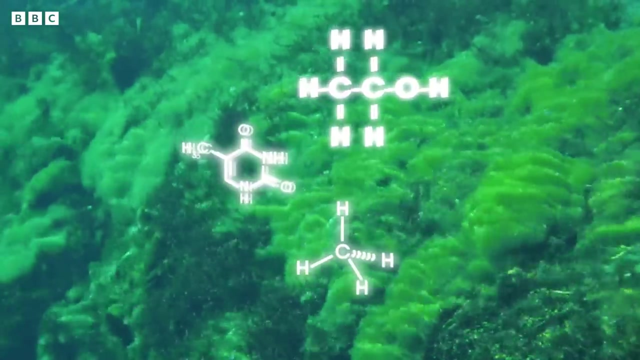 I mean after the investigations of the Galileo spacecraft in the late 90s, Europa became a prime target in planetary science all over the solar system Because with a huge subsurface ocean, with the spectrotidal thermal activity, that became the first place that could be habitable in our solar system besides maybe Mars. That immediately sparked proposals of missions to go back to Jupiter and specifically investigate Europa. I mean, if you are a planetary scientist, probably the most rewarding science goal is to see if a planetary body is habitable or actually inhabited. So Europa Clipper will stay in orbit around Jupiter. 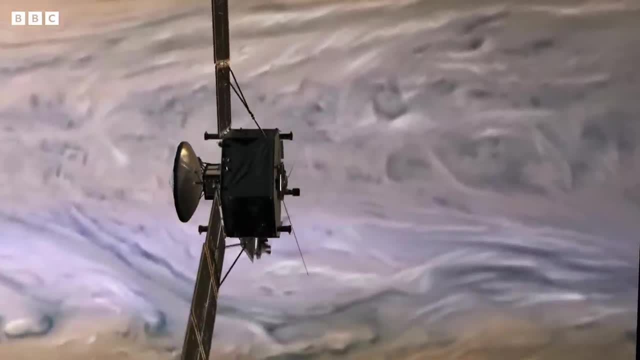 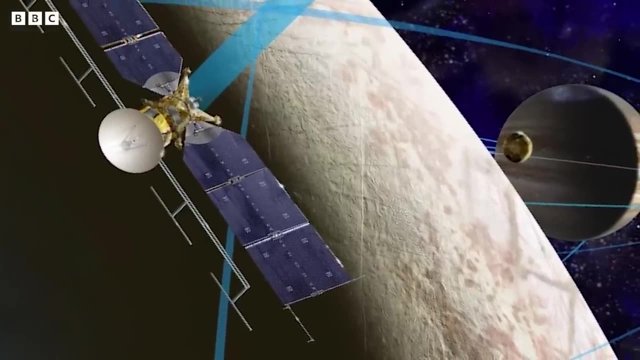 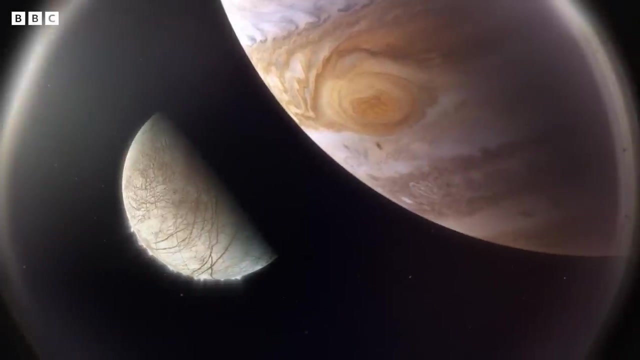 and in most of its revolutions it will have a close flyby at Europa And the flybys are arranged in a way that it's like a web in the end surrounding the Moon, that you have, in the end, a good overview over almost the entire surface after these 50 flybys. 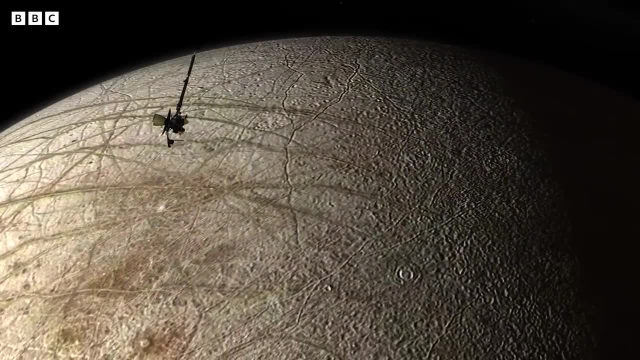 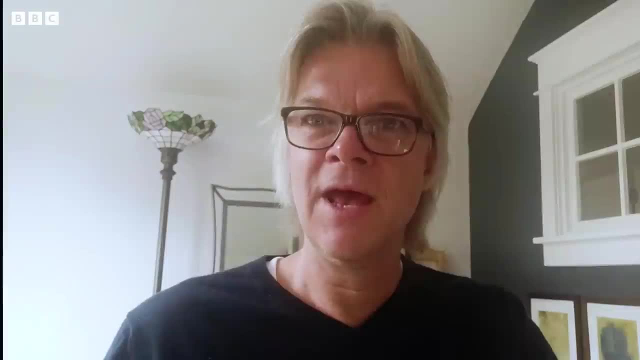 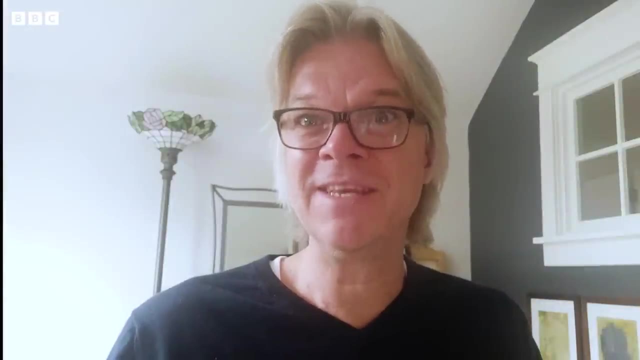 During these close flybys, you get an idea of what is evaporating from the surface of Europa, And from that, of course, you learn about the makeup, the composition of the surface, And this is, of course, specifically true if there is plume and wetting activity. 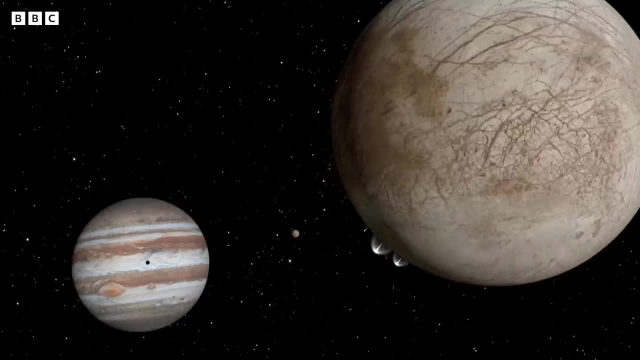 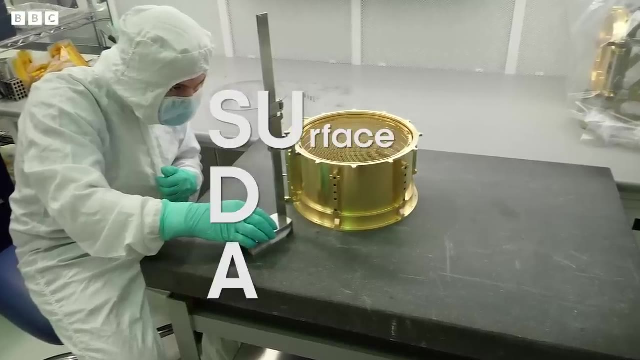 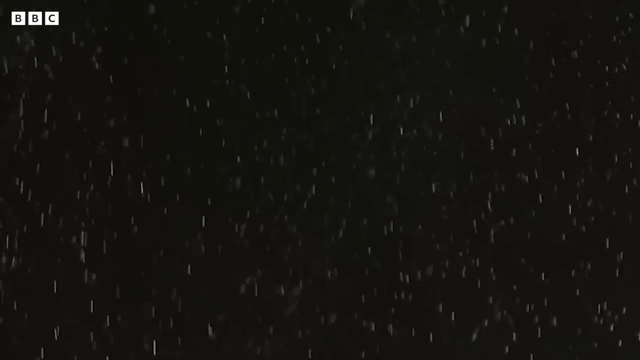 That's what I really would put a smile on my face, if we could measure plume material that's connected to the subsurface ocean of Europa. The instrument called SUDA, the Surface Dust Analyzer, is the instrument I'm working on. It measures the composition of tiny grains that are surrounding Europa. 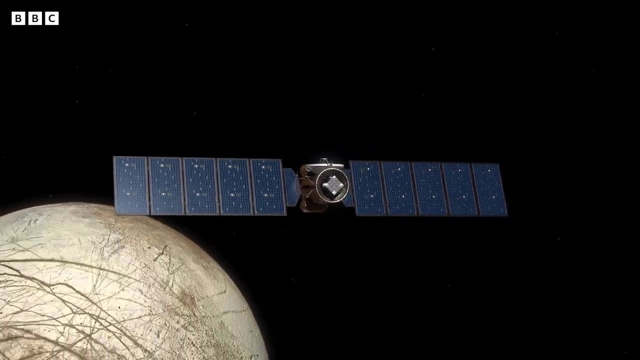 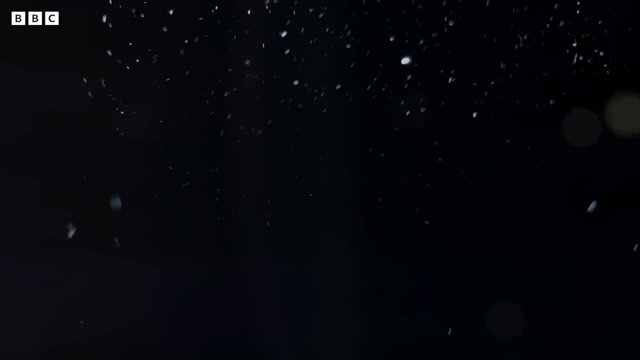 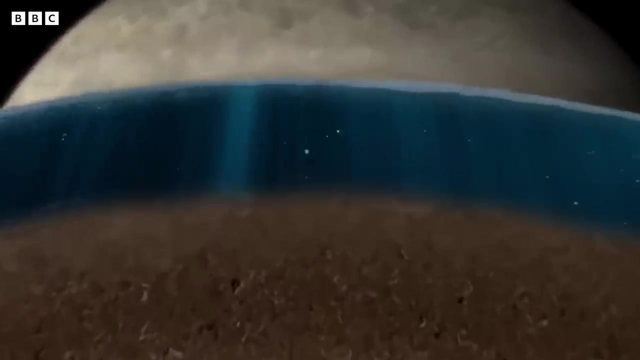 mostly ice grains, And these grains are knocked off the surface due to micrometeoroid impacts. With the SUDA instrument we can sample these materials And with that we get an idea about the surface composition. We could constrain what salts were there in the ocean. 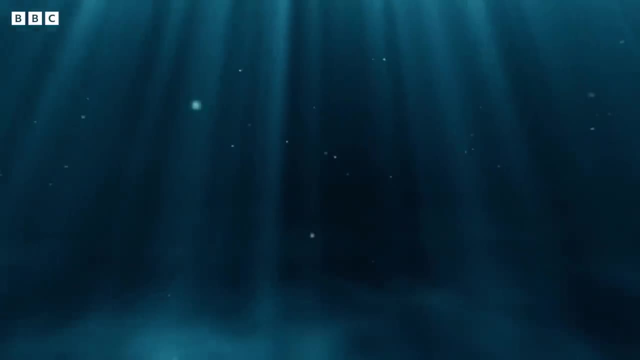 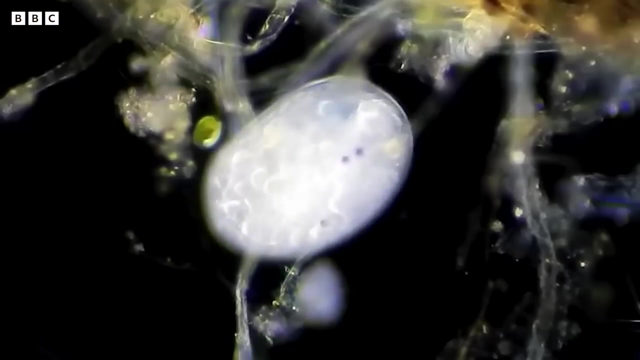 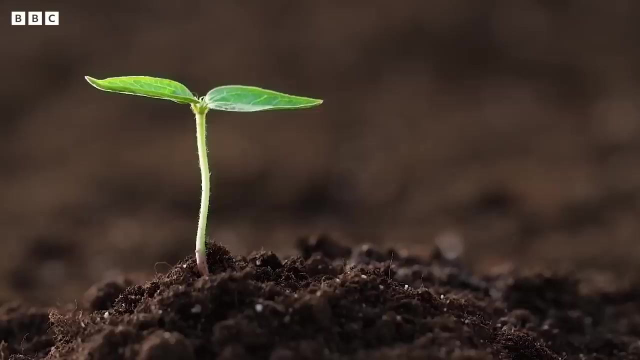 if there's an alkaline, neutral or basic environment, if there's hydrothermal activity at the bottom of the ocean, what the organic chemistry inside the ocean has evolved to? Unfortunately, we currently only have one example of a planetary body or moon where life exists. 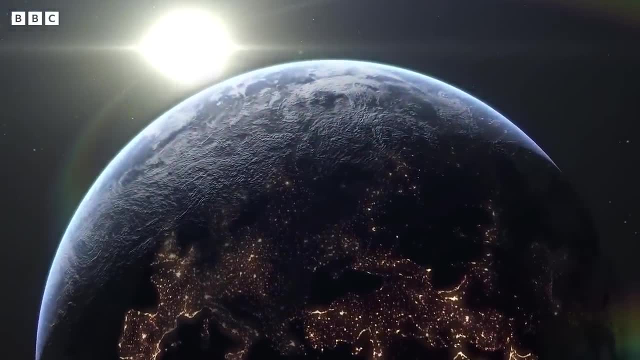 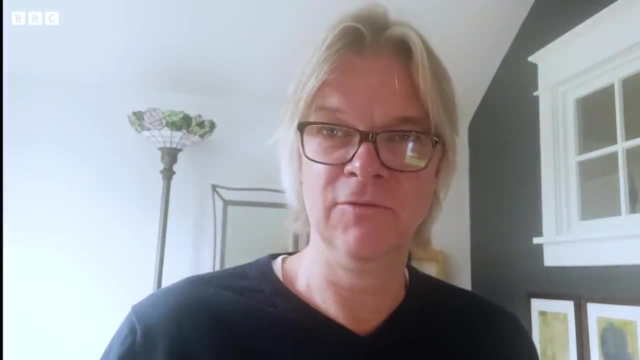 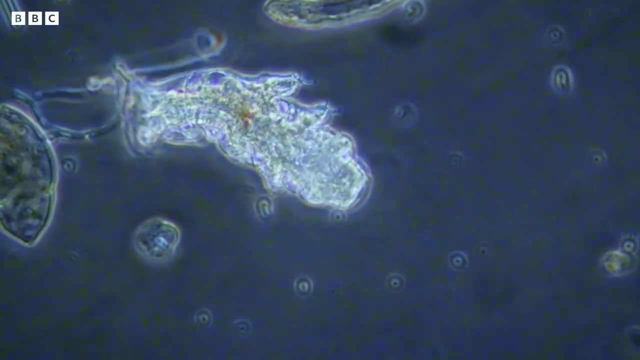 And so it's very difficult to speculate about the nature of life elsewhere. If we look for signs of life on an icy moon like Europa, it's probably most straightforward to just look for simple forms of life If there would be complex civilizations in the subsurface oceans.